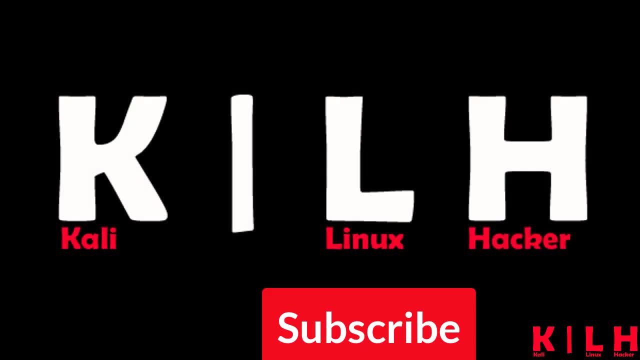 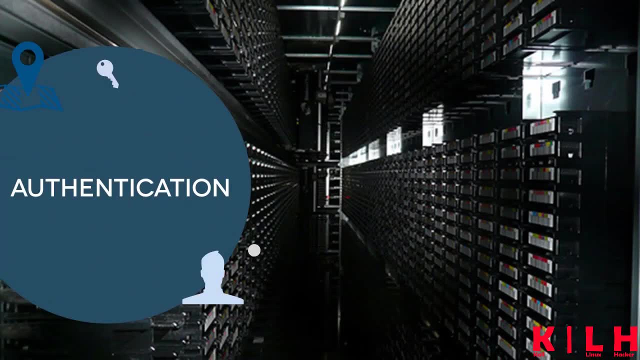 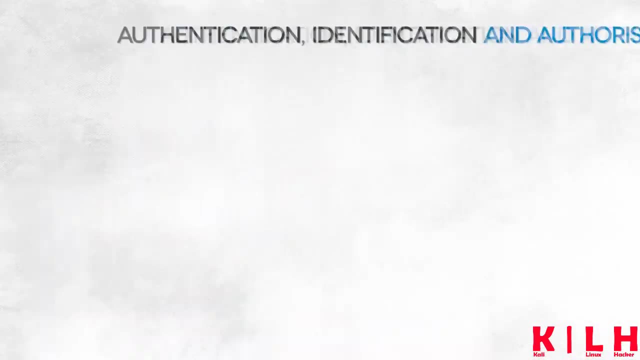 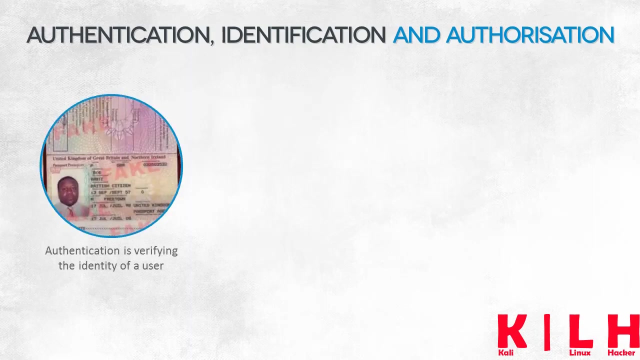 Welcome to a module that will focus on authentication, or in other words, the mechanisms for establishing the identity of users. Let's start off by explaining the involved terms and concepts. Authentication is a process of proving and verifying the identity of a user. You can see an example of authentication evidence in the left side of the slide. 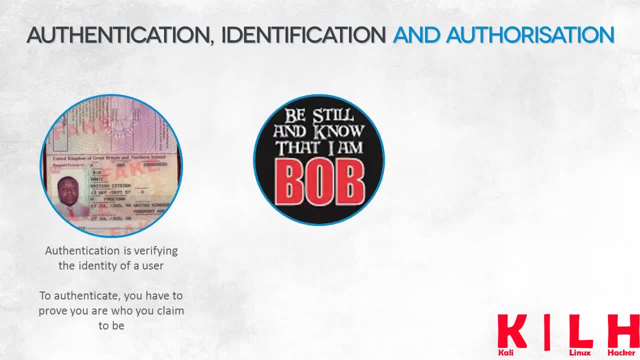 To be able to authenticate someone, you need to have a reason for believing that that person claiming to be Bob is really Bob. A sufficient reason could be an identity document that contains a photograph of its holder or a person who looks like them. This doesn't mean that the person is who they claim to be. 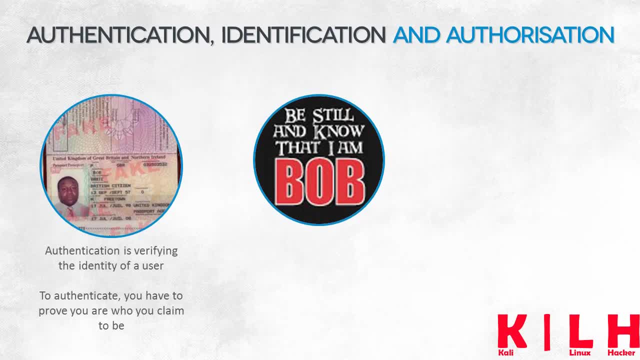 The authenticity of the document should be verified. See if the issuer of the document is on your list of trusted entities. Identification, on the other hand, is, for example, this simple claim: My name is Tom, Nothing else is needed. There is no need to prove or confirm the claim. 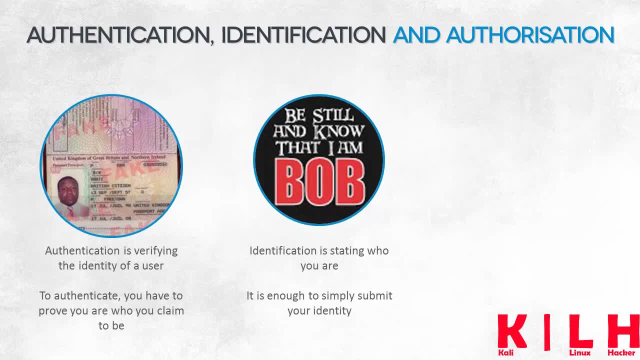 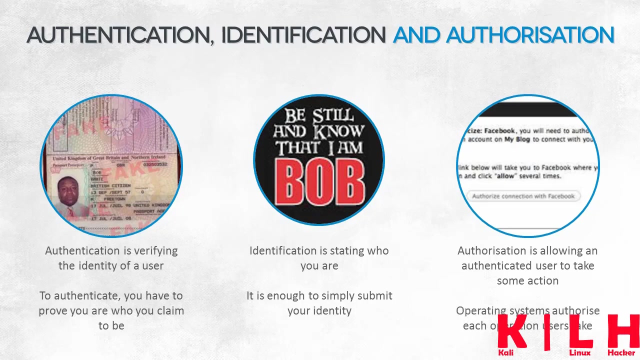 Identification does not equal authentication. Authorization, in contrast to the two above concepts, involves verifying if a person who has confirmed their identity, who is successfully authenticated, has an appropriate level of permissions required to execute an operation. Operating systems usually authenticate users only once at system logon. 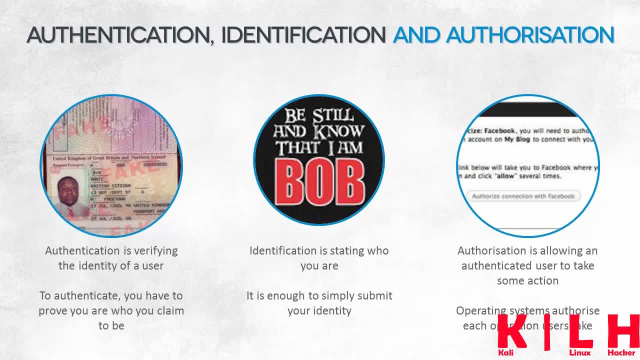 Authorization, on the other hand, is performed each time a user is authenticated. Authorization, on the other hand, is performed each time a user attempts to perform any operation: Run an application, open a document, delete a file, and so on. 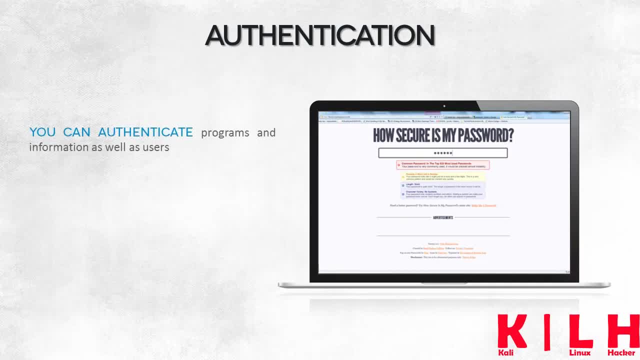 Authentication can be applied to a user or a program, or even to data. The most common method for authenticating users, which will probably remain popular for quite some time, is checking if they know a secret that nobody else should know. This involves checking if a password entered in the login screen is correct. 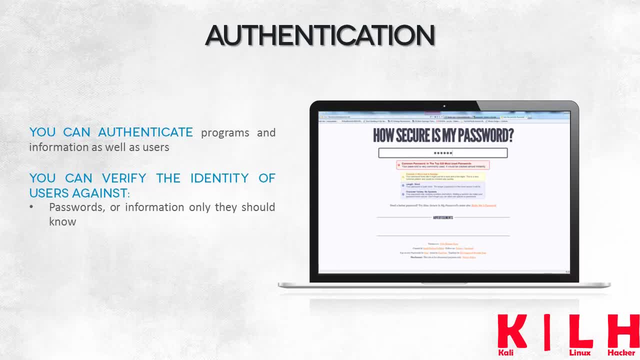 Authentication can also be performed in other ways. You can, for example, authenticate a principal, a person, by ensuring they possess some data that is exclusive to them. This type of information is usually saved in private keys or stored on smart cards. We'll go back to smart cards later. 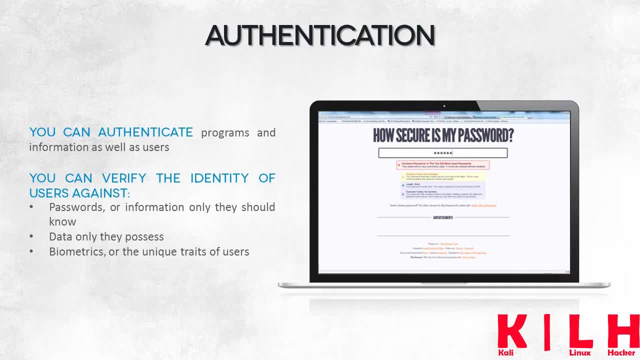 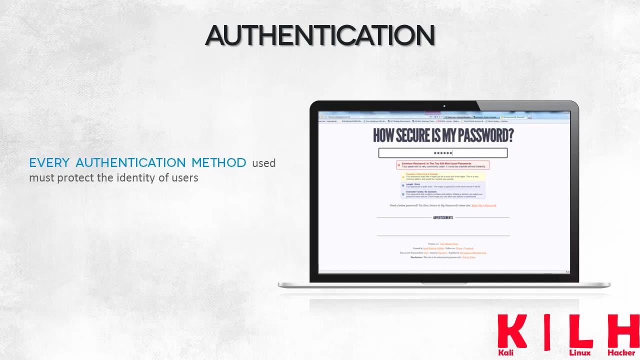 Biometric authentication is another solution. Biometrics is based on a person's distinctive features. Modern operating systems can implement the use of all three techniques, either separately or together. The most common method is password authentication, which we'll look into more closely in a moment. 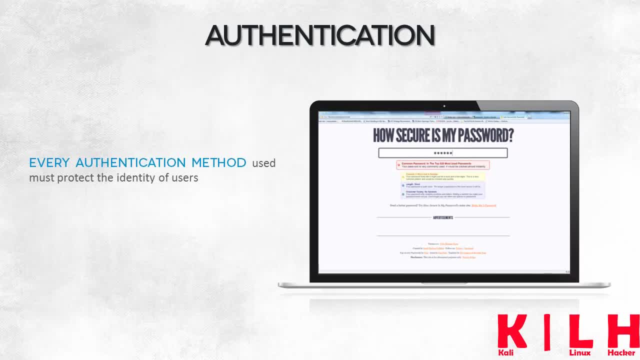 Smart cards authentication is also very popular. Many computers, including portable computers, are equipped with biometric readers. They're less popular, however, and one could claim that they're less effective. Authentication is a process of proving an identity with the use of a secret. 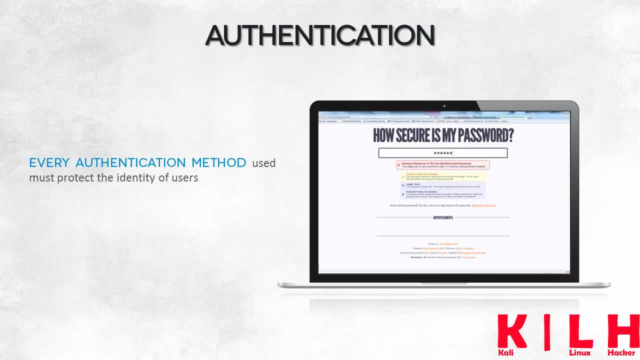 If something is to remain secret, it has to be changeable. We should change our passwords more or less regularly. It's also easy to issue a new certificate or renew an existing certificate. It's harder, however, to replace a hand or an eye. 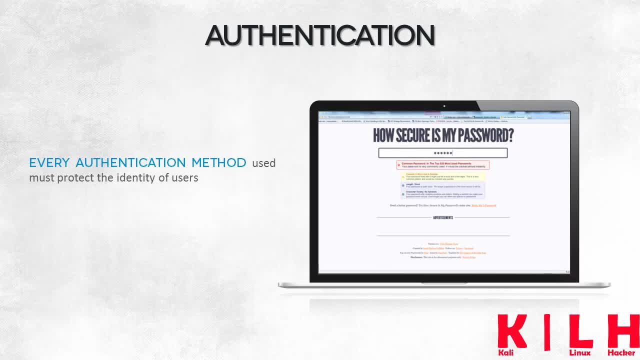 It could happen as well- perhaps not too often- that employees will travel to places where bodily integrity is low on the priority list for local criminals. Coercion can make you give away your password or hand over your smart card. It's harder, however, to persuade someone to part with their finger or eyes. 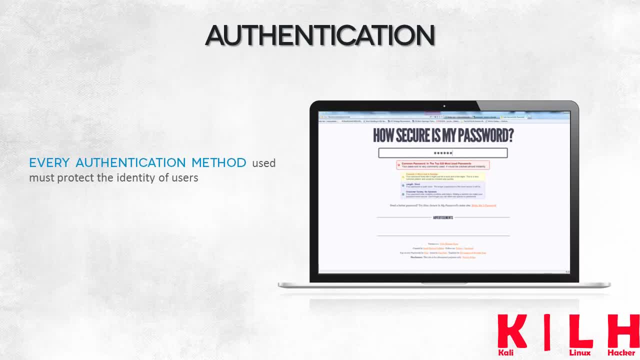 It doesn't make sense to implement authentication methods that only provide further threat to users. Let's return to passwords for a moment. The problem with passwords is that, with time, computers are running faster and faster. A password that was secure ten years ago: eight characters, including alphabetic, numeric and special characters. 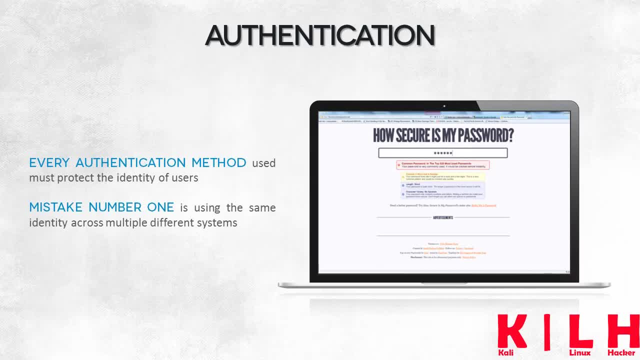 has decreased on the security scale. To catch up with increased computer performances, user passwords would have to be ever longer. We'll show this in a minute. Longer passwords mean more trouble with remembering them. A 64-character random password is practically impossible to remember. 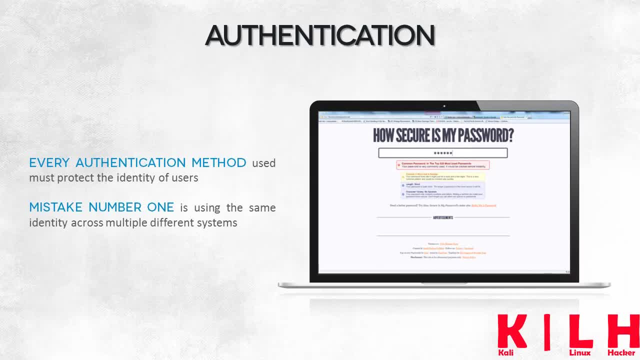 And even if you do memorize it, you're sure to make typos entering it. That's why implementing additional authentication is crucial. Since we've mentioned that biometrics is not an ideal solution, we're left with smart cards. The advantage of smart cards is that they can store large amounts of data. 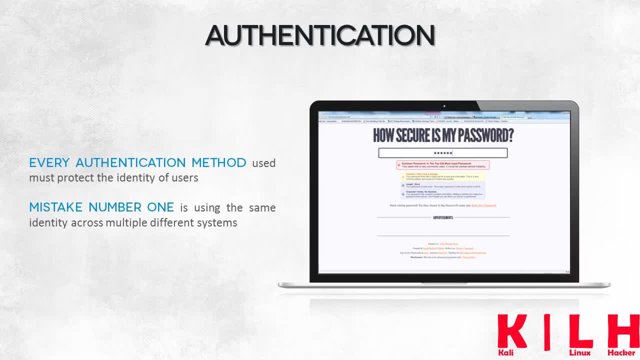 which means that passwords and keys can be long and we don't have to remember them as well. This is the main strength of smart cards. Announcing that your company will implement two-factor authentication could also bring some unexpected benefits. This was the case with Microsoft Corporation. 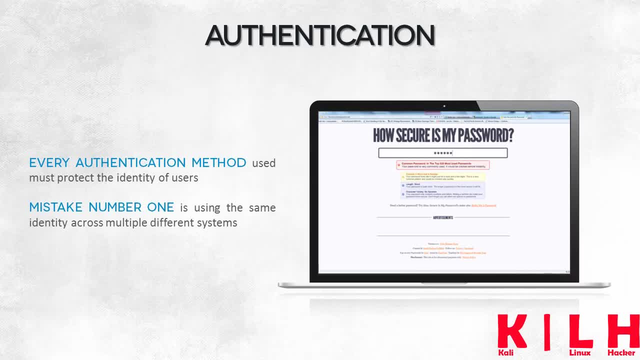 Some time ago, 20-30% of traffic at parameter routers in Microsoft networks was made up from attempts to crack staff passwords. Usually, the attempts failed, but even ignoring the potential threat to security, cracking attacks were an infrastructure issue. The network slowed down as a result. 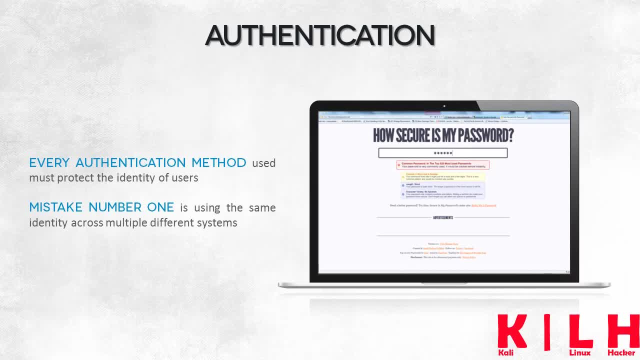 Microsoft announced that they'll also use smart cards, in addition to passwords, to log onto a computer. This makes cracking a password impossible without physical access to the card. This is the second authentication factor. One is something the user knows: a card's PIN. 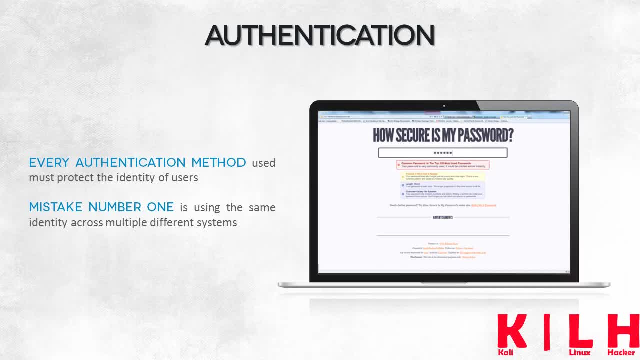 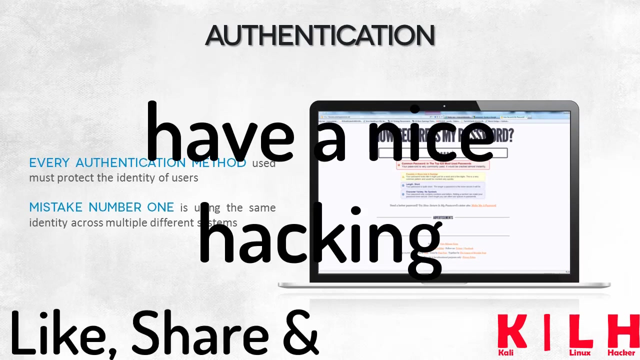 Second something: the user has data saved in a card. Most attackers, except for the ever-optimistic types, stopped brute-forcing Microsoft passwords. The network sped up without any infrastructure development. The solution is easy and effective. Thank you.